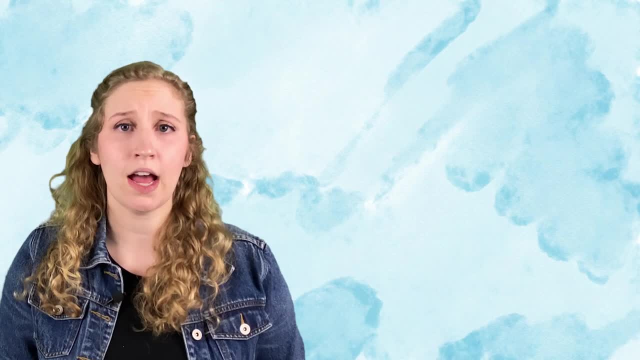 right here, which is a virtual protractor. We're going to break it down in just a few seconds. So we're going to break it down in just a few seconds. We're going to break it down in just a few seconds. So we're going to break it down in just a few seconds. 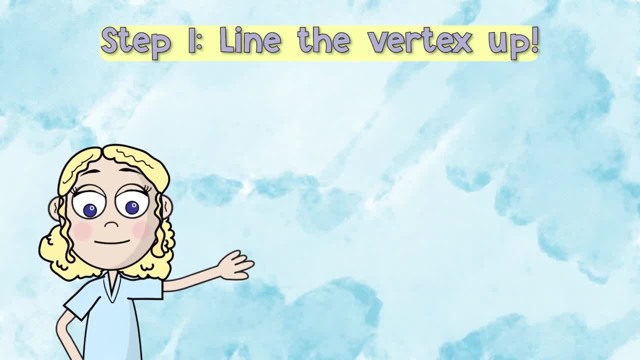 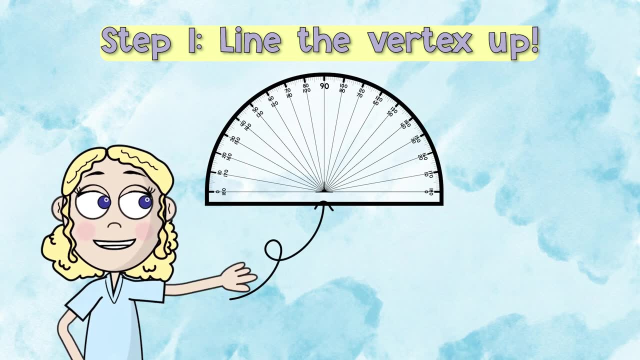 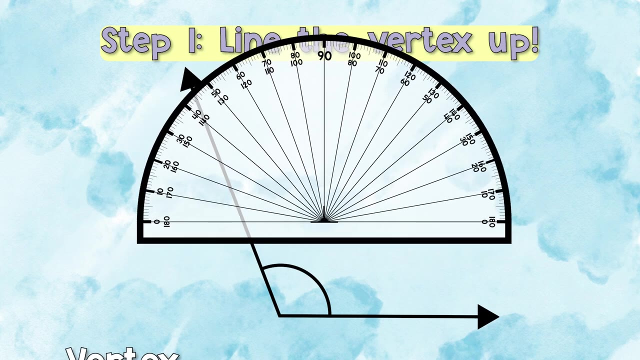 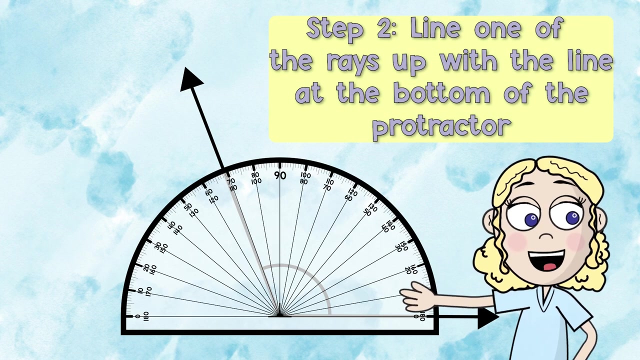 into a few steps. Step one: you are going to put the whole circle or dot on your protractor so that it's lined up with the vertex. This might also look like a little upside down T. Step number two: you will then line up one of the rays. 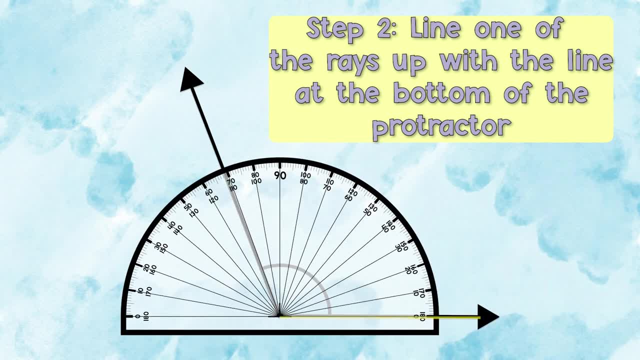 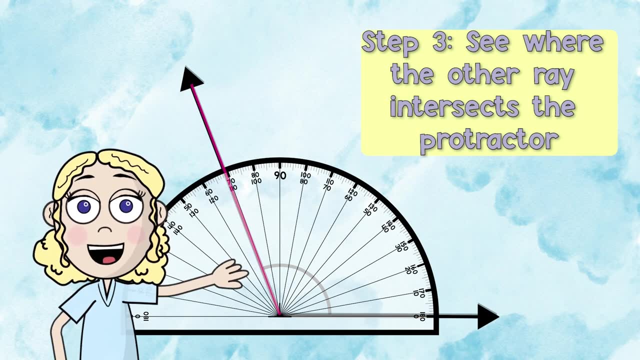 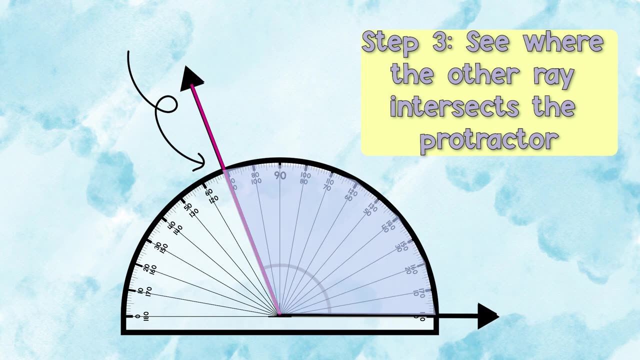 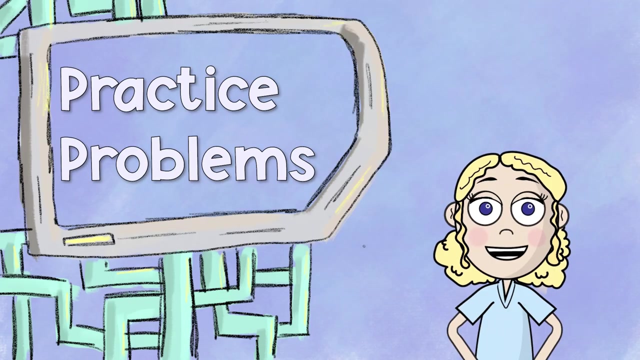 with the line on the bottom of the protractor, Step three- you will see where the other ray intersects the protractor, and that is where you will find your ankle measurement. That's how you measure. hooray, All right, now that you know how to measure. 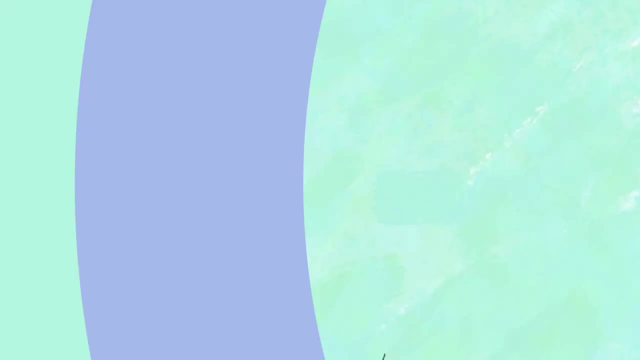 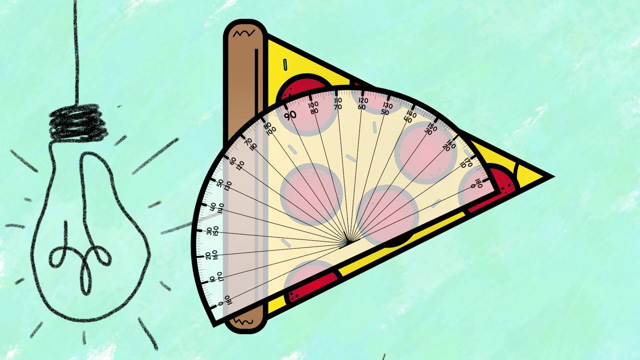 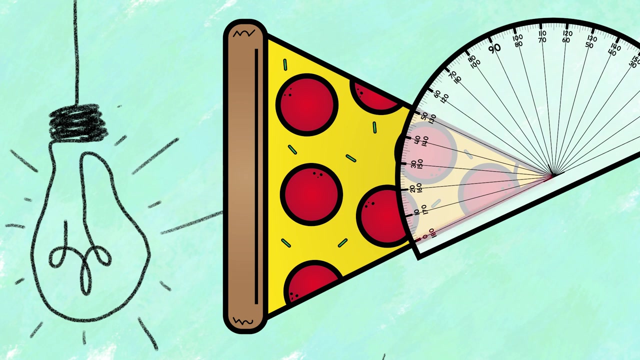 let's try a few practice problems. Let's look at this pizza. Step one: we're gonna line up the dot circle, or T, on the vertex. Step two: we're gonna line up the one ray with the bottom line on the protractor. 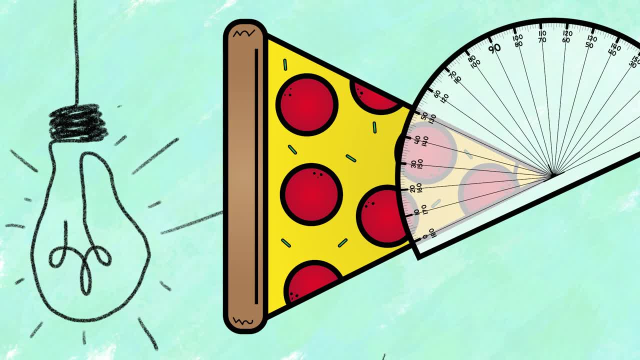 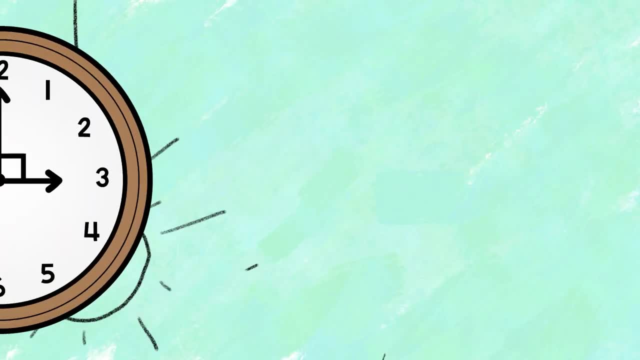 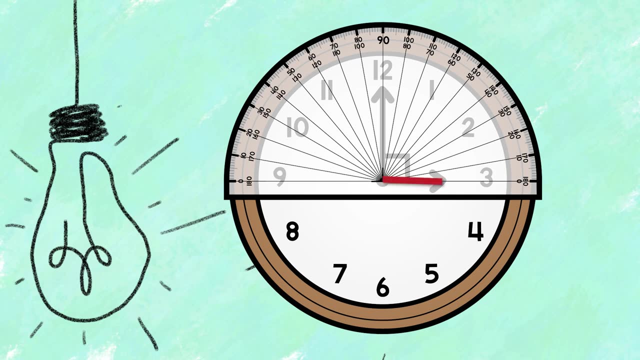 Step three: we are going to look at where the other ray intersects Ta-da. All right, now let's look at this angle. Same thing, step one: line it up on the vertex. Step two: bottom line with the ray. 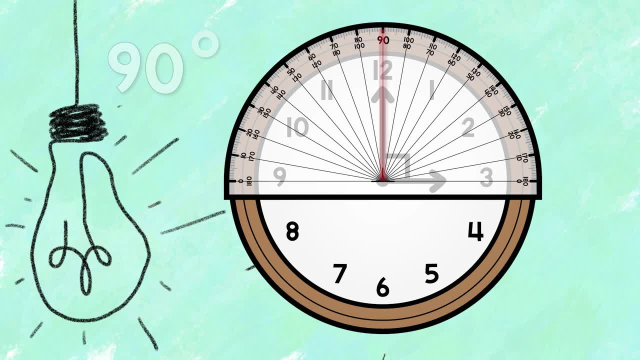 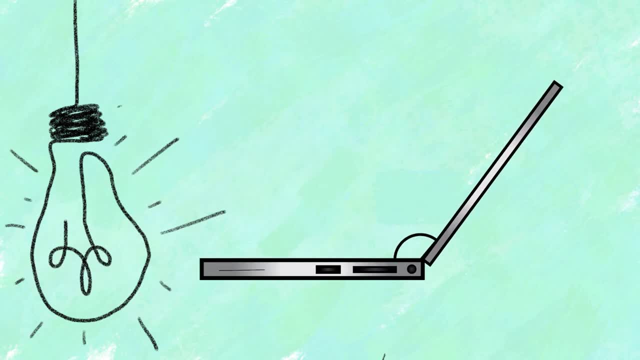 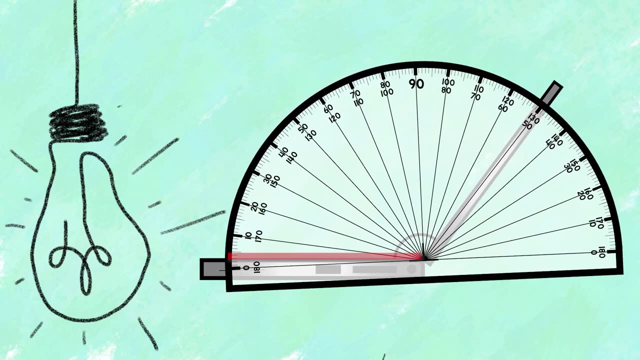 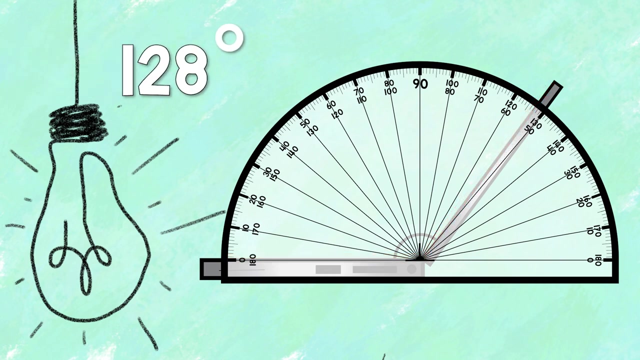 Step three. where does the other line intersect, Ta-da? All right, last one, Here we go again. Step one, do you remember? Step two, step three, And here is our measurement in degrees of this angle. All right, 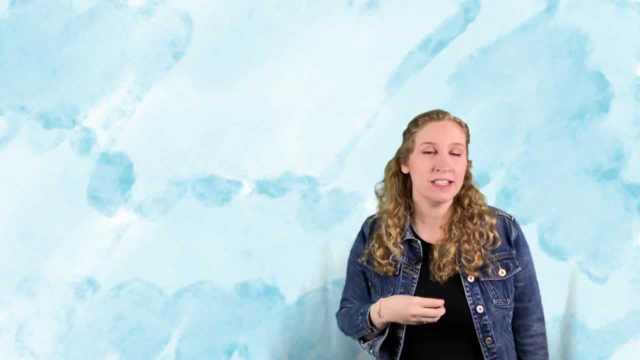 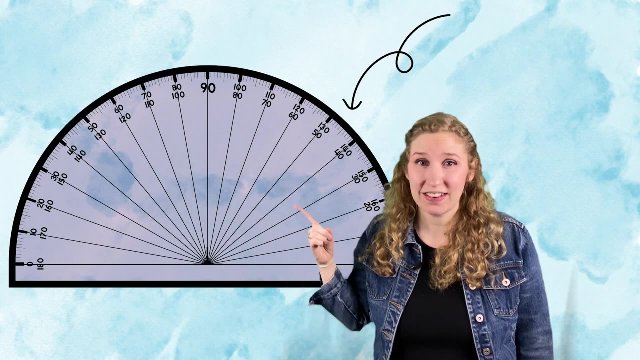 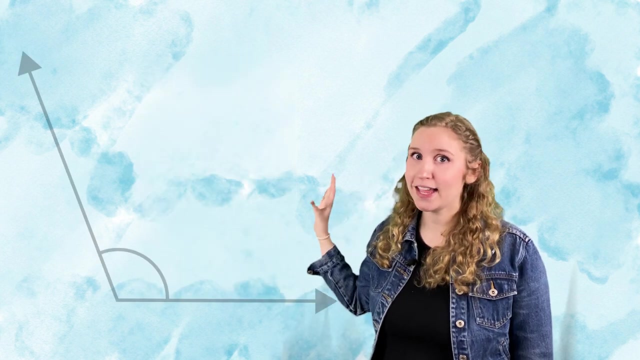 All right, Here's a trick. If you know the different types of angles- acute, obtuse, right- you can actually use that to estimate and figure out which set of numbers you need to use and also check your thinking. So, for example, if you're measuring this obtuse angle and you see,